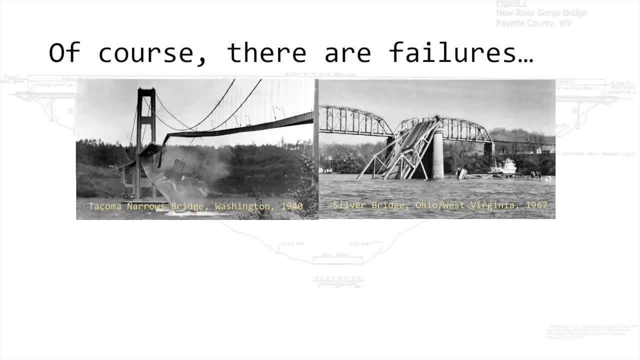 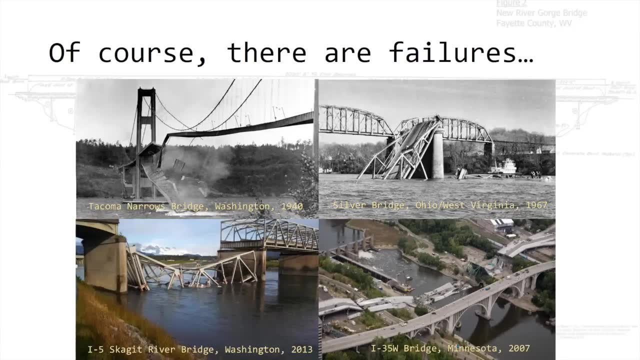 Are bridge failures just a thing of the past? Unfortunately, the answer is no. More recent failures include the I-35 West Bridge in 2007 and the I-5 Skagit River Bridge in 2013.. Failures are never desirable. 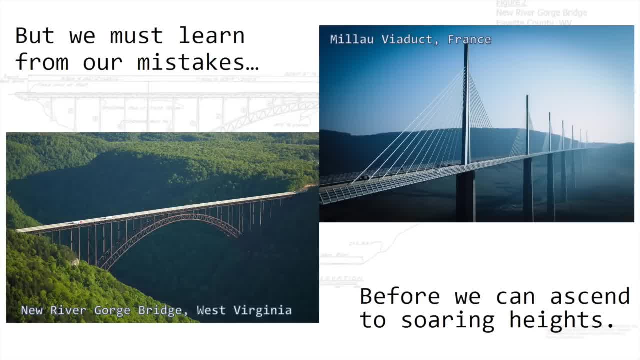 But through failures we learn how to design better bridges. Why do you think bridge failures are so insightful? When a design works, we may not always know exactly why it works, but we continue to use the design. When a design fails, the reason for failure becomes evident, which leads us to a better understanding of the physics of bridge designs. 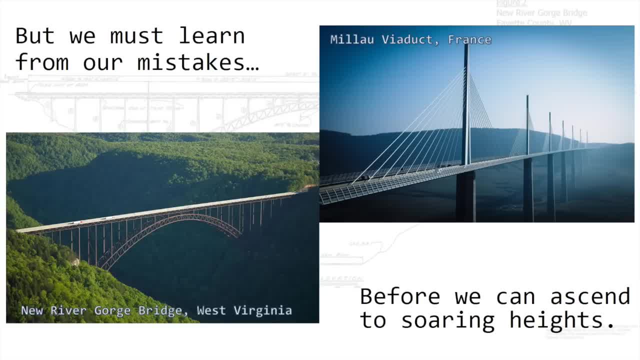 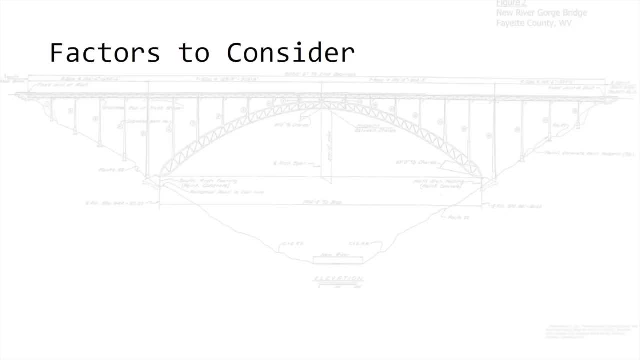 Increased understanding leads to incredible achievements like the New River Gorge Bridge and the Malau Viaduct. What are bridge engineers? Bridge engineers must consider six factors in developing designs. What do you think these factors are? The first question is always one of function. 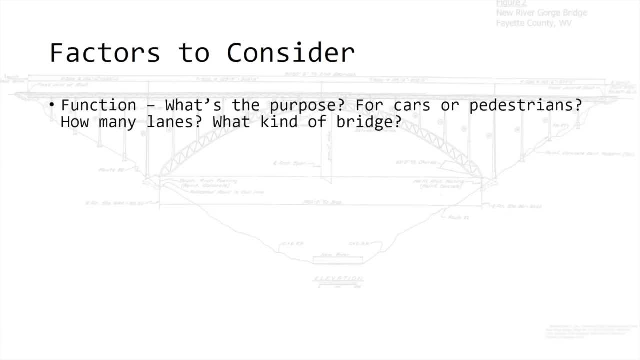 What's the purpose of the bridge? Is it for vehicles or pedestrians? How many lanes are needed? What kind of bridge should be designed? After function comes the question of materials. What kind of materials should be used to construct the bridge? The answer to this question usually depends on the bridge type and site conditions. 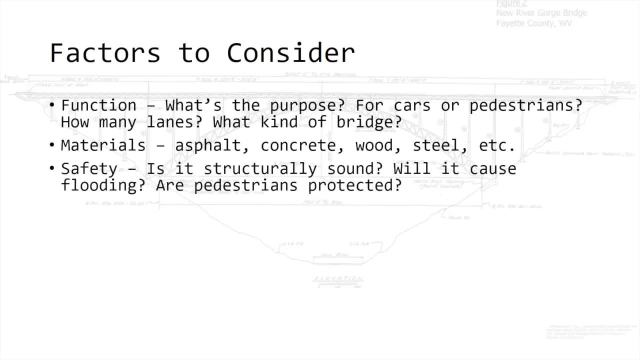 A very critical question then comes into play: Safety. Is the bridge structurally sound? Has it been designed for an appropriate factor of safety? Will it cause flooding? Will pedestrians be protected? These questions are all answered during the design phase. Once designs have been drawn up, the cost of the designs must be considered. 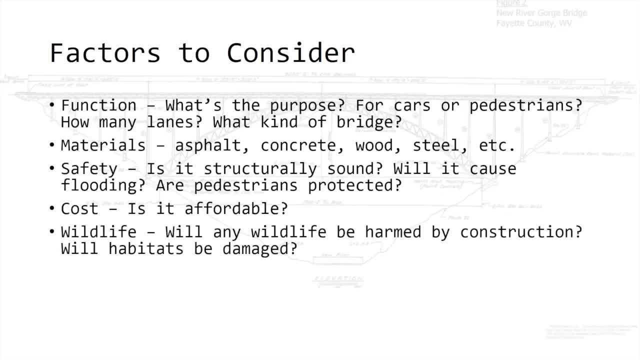 Costs can be monetary, But impacts to wildlife must also be considered as a cost. Any time wildlife is harmed or habitats are damaged, the project has incurred both economic and ecological costs. Finally, the question of appearance is also asked. Is the bridge aesthetically pleasing? 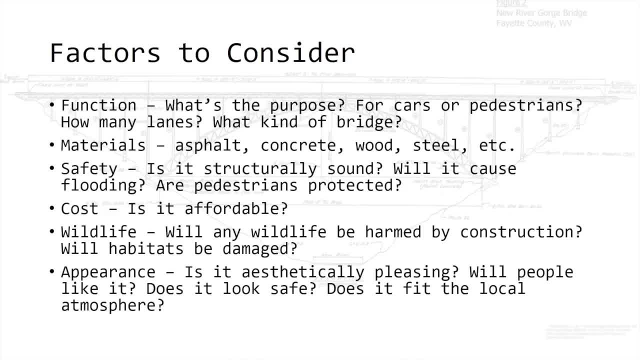 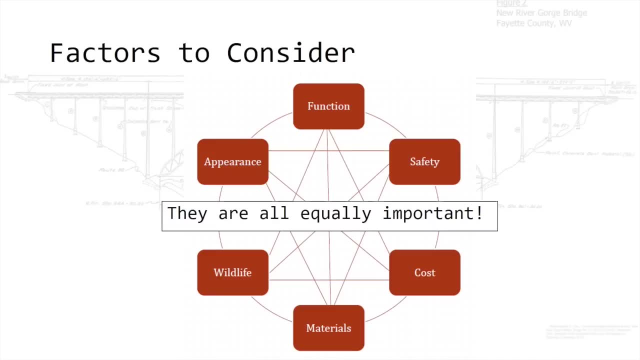 Will people like it? Does it look safe? Will it fit with the surrounding atmosphere? Of these six factors, which do you think is the most important? All of the factors are equally important, because all of the factors are intertwined. The best design is one that satisfies each of the six factors. 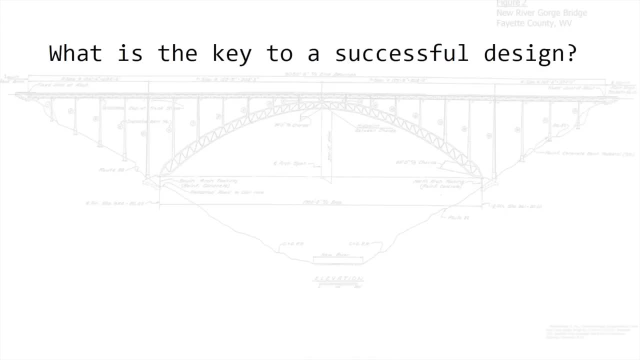 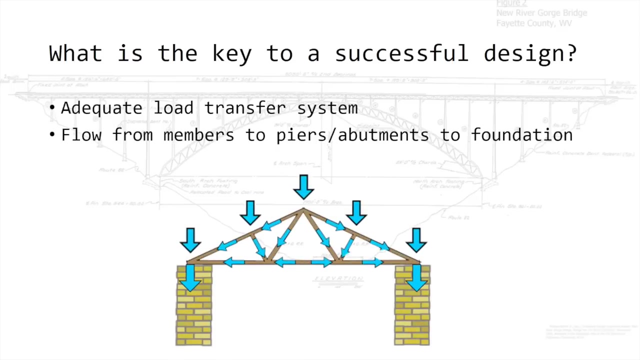 Let's turn our focus now to the safety aspect of design. What is the key to a successful design? A successful design must be able to adequately transport from the structural members to the piers or abutments and finally into the foundation and the ground. 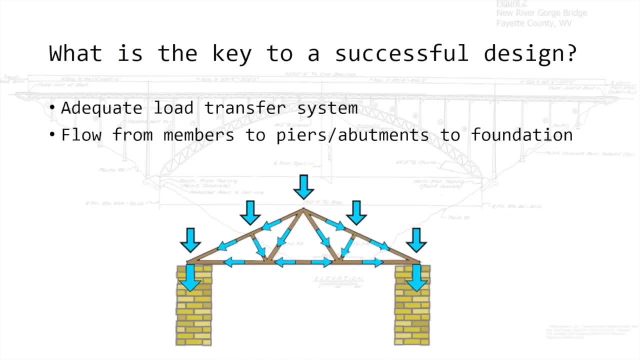 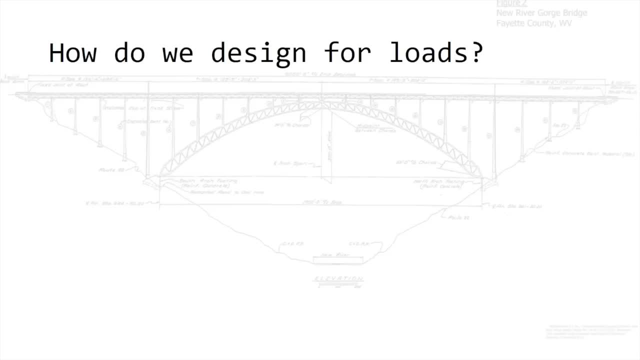 How do we design for loads? We apply Newton's second law, which states that the net force equals mass times- acceleration, But bridges aren't moving. So what happens to our equation? We apply Newton's second law, which states that the net force equals mass times- acceleration. 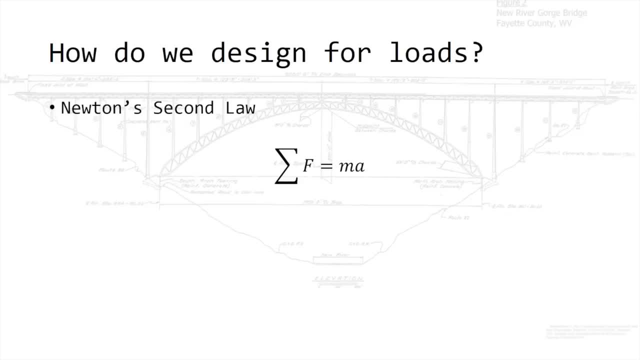 But bridges aren't moving. So what happens to our equation? Since there is no motion, acceleration is zero, which means the net force acting on the bridge must sum to zero. This is a statement of static equilibrium. We have three equilibrium equations that we apply when designing bridges. 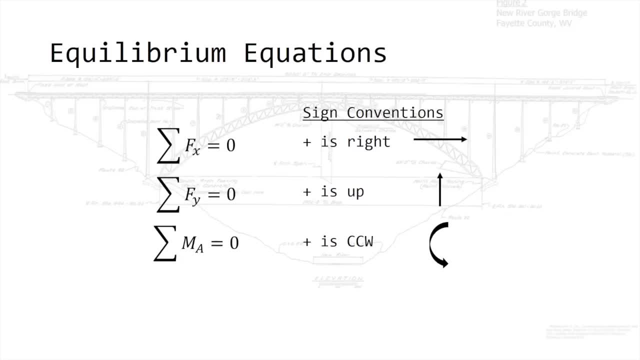 The sum of the forces in the x direction equals zero, the sum of the forces in the y direction equals zero and the sum of the moments about any point equal zero. For each equilibrium equation we have sign conventions for the direction of the forces or moments. 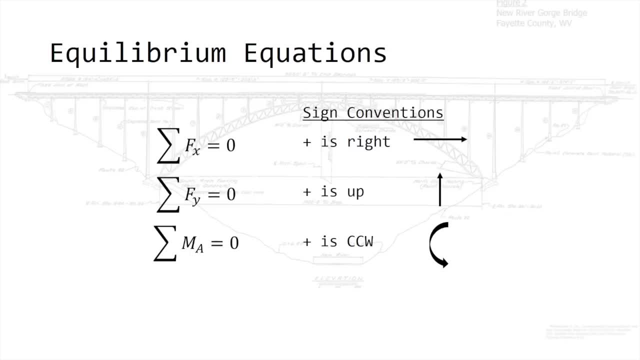 Remember that forces are vectors, so both direction and magnitude need to be accounted for in our equations. In the x direction, positive is to the right. In the y direction, positive is up, And for moments positive is counterclockwise. 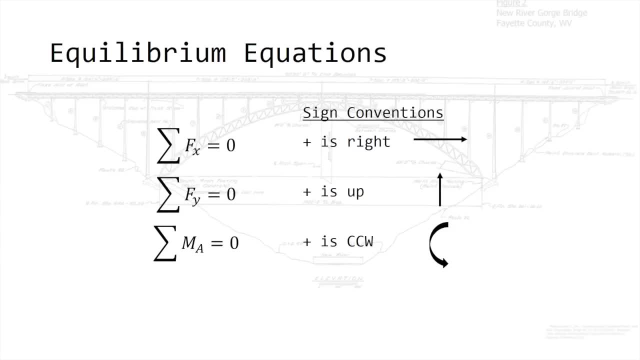 Notice that moments are given directions of clockwise or counterclockwise, because a moment is the rotation caused by a force that is located a certain distance from a point. Moment is given by force times: distance from the point to the location where the force is acting. 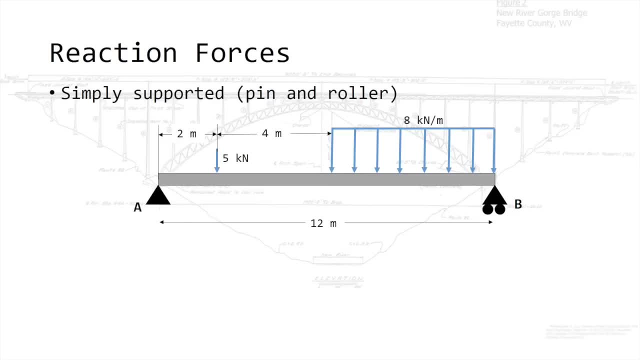 Let's try to apply these equilibrium equations to solve for the reaction forces on this simply supported beam. Simply supported means that restraint is provided through a pin at one end and a roller at the other. Bridges are typically designed as simply supported structures. What kind of movement do you think a pin constrains? 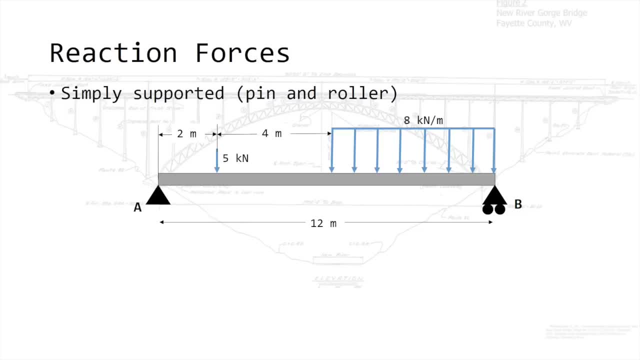 What about a roller? Pins constrain movement in the x and y directions, so we have two reaction forces at a pin. Ax and Ay. Rollers only constrain movement in the y direction, so we have a single reaction force at the roller By. 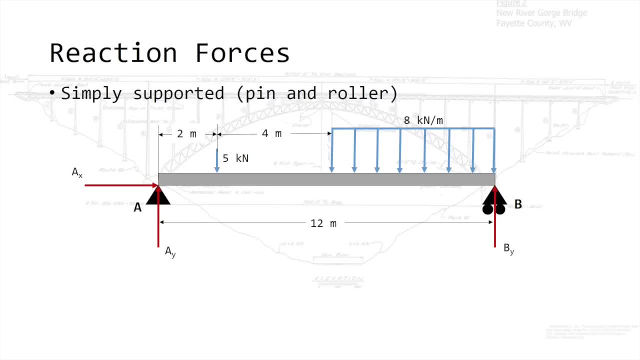 Now we can write our equilibrium equations and solve for the reaction forces: Ax, Ay and By The sum of the forces in the x direction equals zero, which is equal to Ax, since it is the only force we have acting in the x direction. 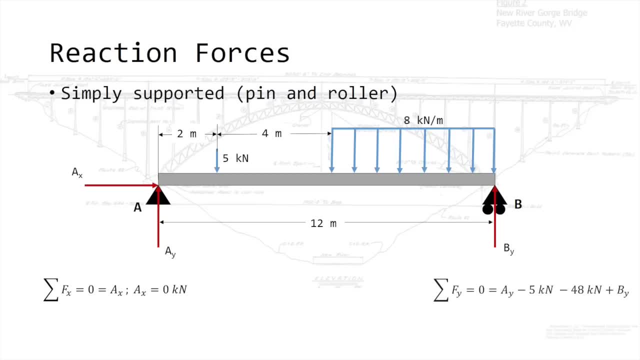 The sum of the forces in the y direction equals zero, which equals Ay minus 5 kN minus 48 kN plus By. Let's take a minute to look at the sign conventions before we move on. Ay is pointing up, so it's positive. 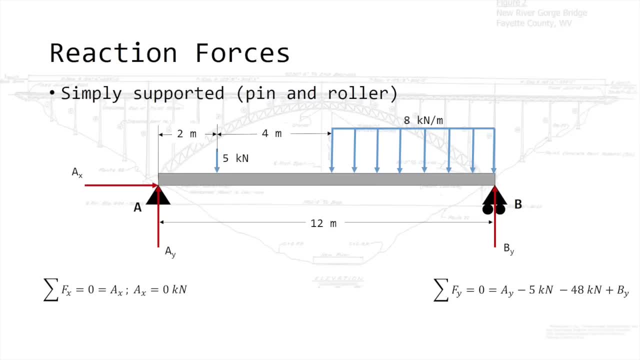 The 5 kN force is pointing down, so it's negative. The 8 kN per meter distributed load can be treated like a 48 kN point load, which is also negative. Finally, By is pointing up, so it's positive. 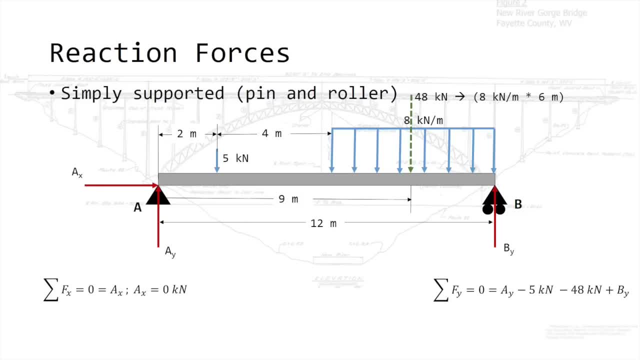 We can't solve this equation because we have two unknowns, so we need to write our third equation for the sum of the moments about a point. Which point should we choose to take the moments about? We should choose a point that will eliminate one of the unknowns, Ay or By. 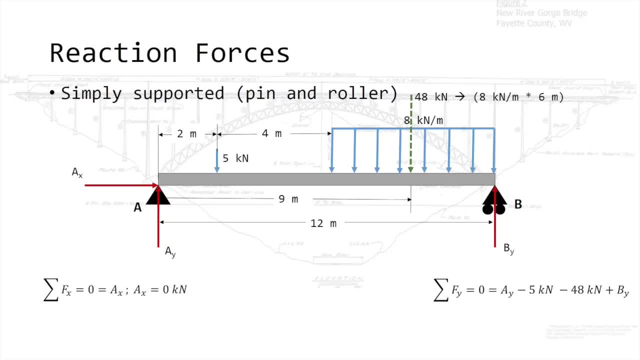 We can eliminate an unknown from the equation by taking the moment at a point that the unknown force goes through. For example, if we take the moments about point A, knowing that moment equals force times distance means that the moment caused by force Ay at point A. 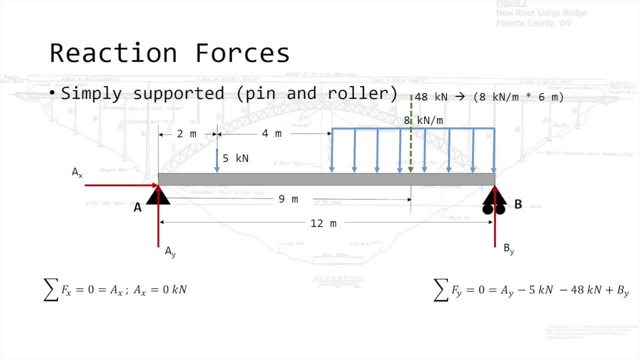 equals zero because the distance is zero. Let's finish writing the equation for the sum of the moments about point A. The moment caused by the 5 kN force is given by 5 kN times 2 meters, Since this force creates a clockwise rotation about point A. 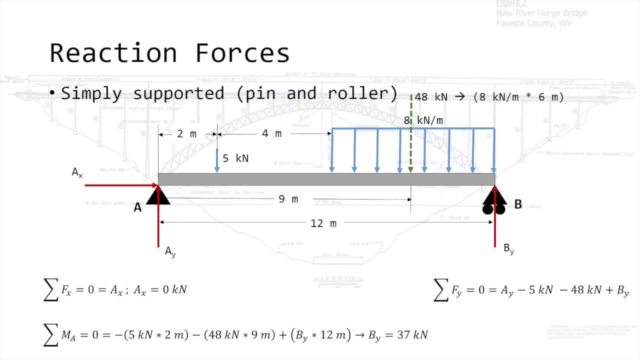 we write it as a negative in the equation. Similarly, the 48 kN force that represents the distributed load creates a negative moment with a magnitude equal to 48 kN times 9 meters. Then last we have By times 12 meters. 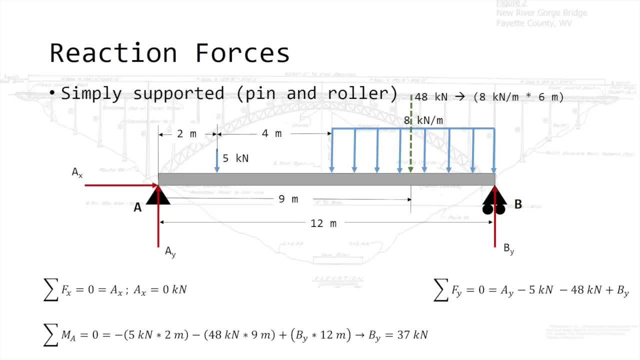 which is positive because it creates a counterclockwise rotation about A. Now we can solve the equation for By which we find to be approximately 37 kN, If we plug this value into our sum of the forces in the y equation. 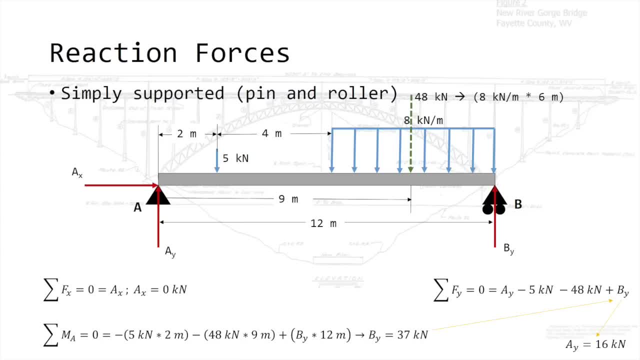 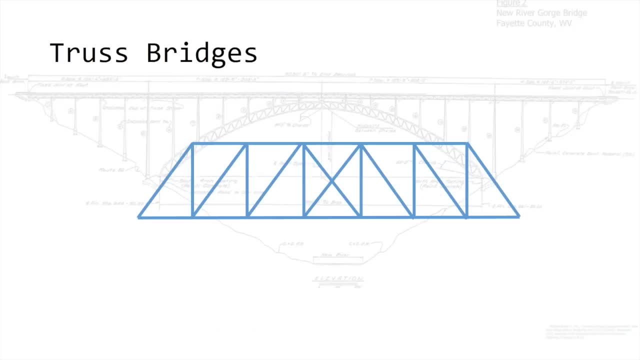 we can solve for Ay, which we find to be 16 kN. Now we've finished solving for the three reaction forces. At the end of this video lecture, you will be constructing a truss bridge, so let's discuss truss bridges specifically. 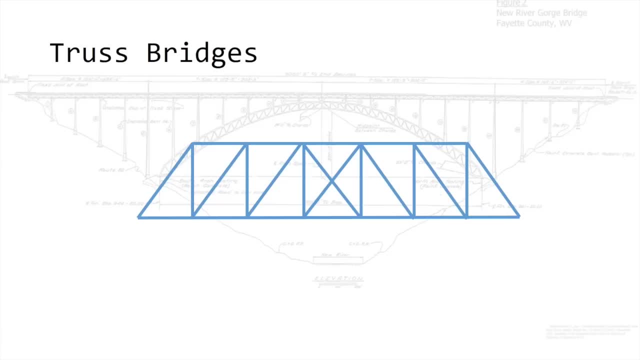 Truss bridges can be constructed from steel or wood and the members are placed in triangular configurations. Truss bridges have five main components: The bottom cord, the top cord, the diagonals, the verticals and the joints. Trusses are called non-load path redundant structures. 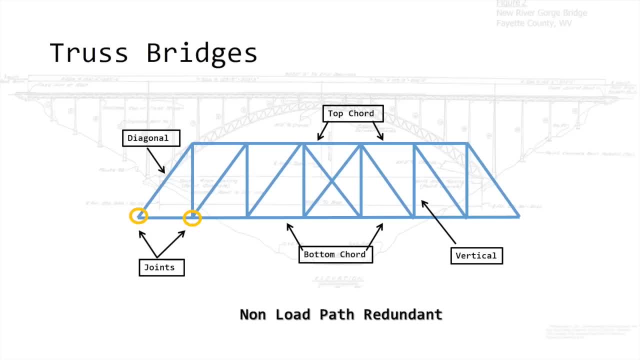 because if a certain member fails, the entire bridge will fail. These members, called fracture critical members, are a key part of the load transfer system, because there is no other load path for the forces to flow through if only a single fracture critical member is missing. 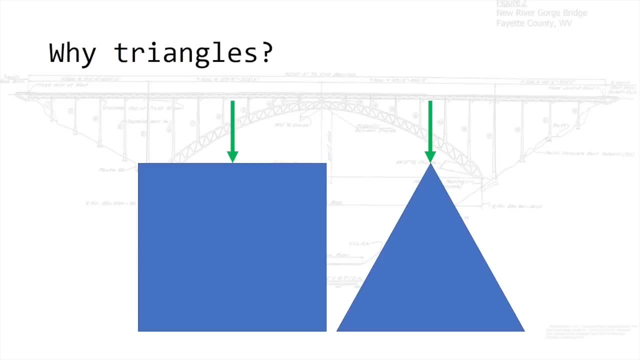 So why do you think truss bridges and triangles are chosen in design instead of squares? If we apply the same load at the top of a square and a triangle, what do you think will happen to each shape? The square deforms under loads. 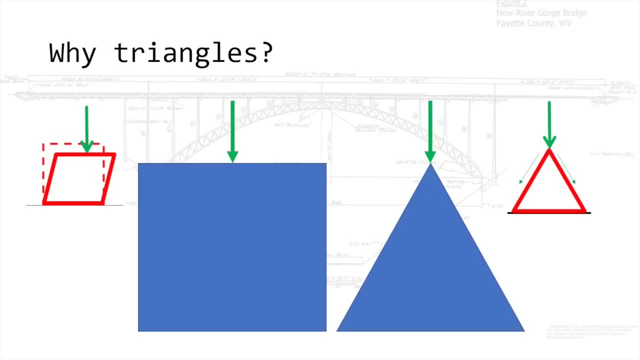 while the triangle maintains its shape and allows the forces to flow through the sides and into the ground. How do we know what forces are being carried by the triangles in the truss? To answer this question, we have to complete a truss bridge analysis. 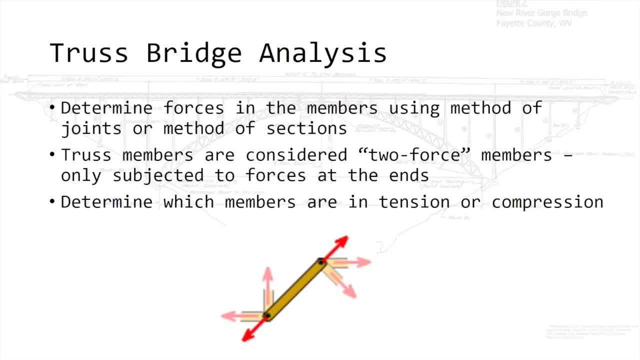 This analysis involves applying three equilibrium equations to determine the forces in each member, using either the method of joints or method of sections. Truss analysis assumes that the members are two force members, meaning that members are only subjected to axial forces at the ends When we calculate the forces during analysis. 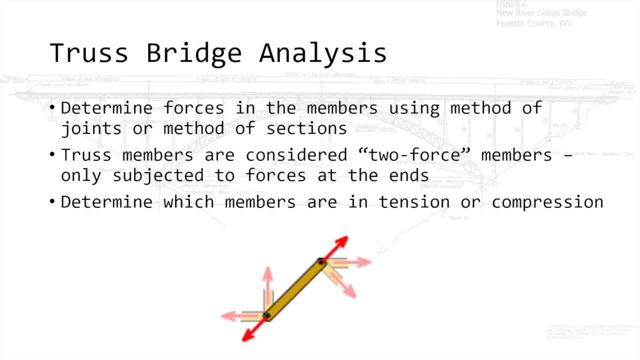 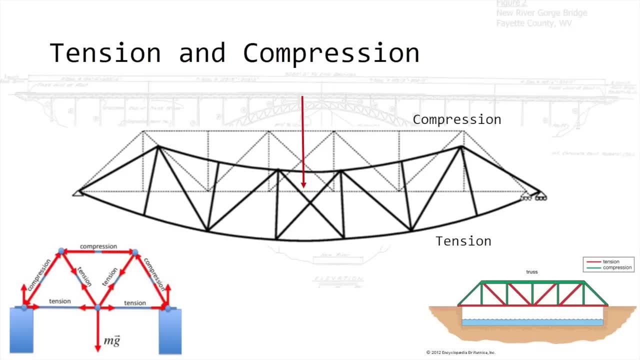 we also find out whether the forces are causing tension or compression in the member. In general, when the bridge is loaded, it's a form such that the top is in compression and the bottom is in tension. We can intuitively decide that the top chord members will have compression forces. 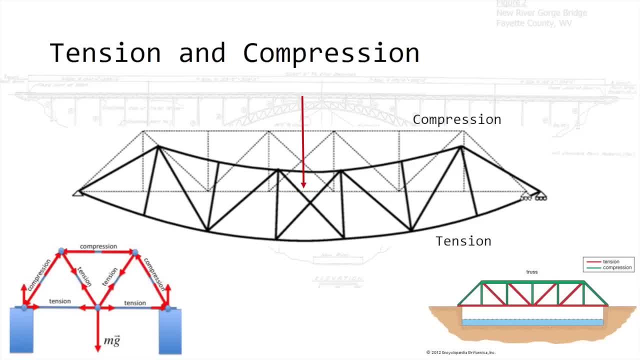 and the bottom chord members will have tension forces. Whether the rest of the members are in tension or compression will be evident during the calculations. Negative forces signify compression and positive forces indicate tension. The tension compression assumptions for the bottom and top chord members can also be checked during the analysis phase. 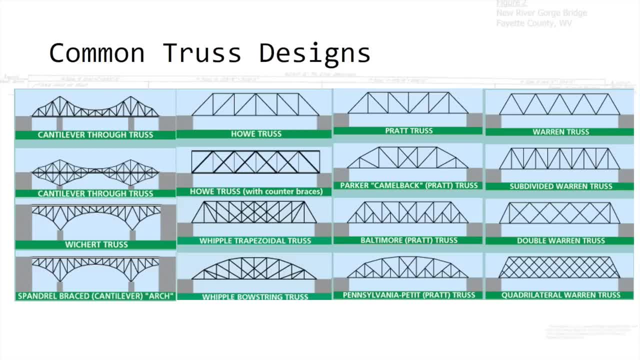 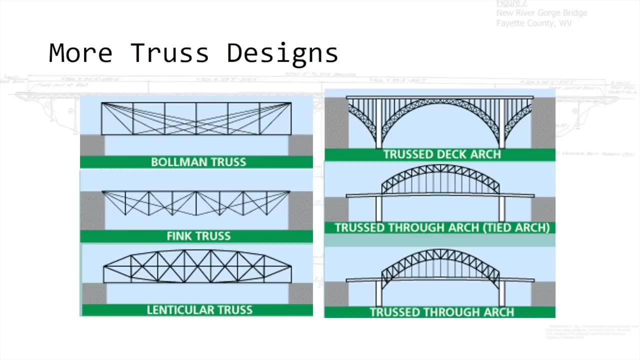 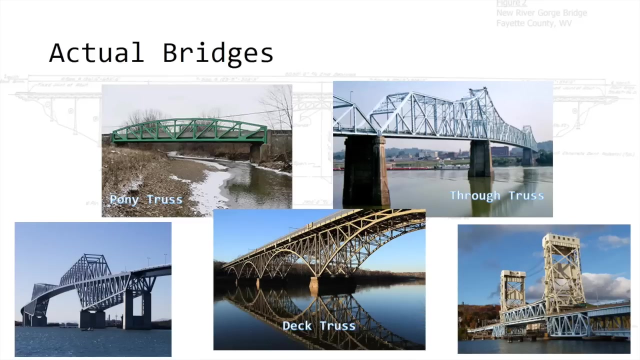 Trusses can take on a variety of different designs depending on the configuration of the triangles. You might be familiar with some of these common designs, But other, less traditional truss designs also exist. We can see these designs show up in actual truss bridges. 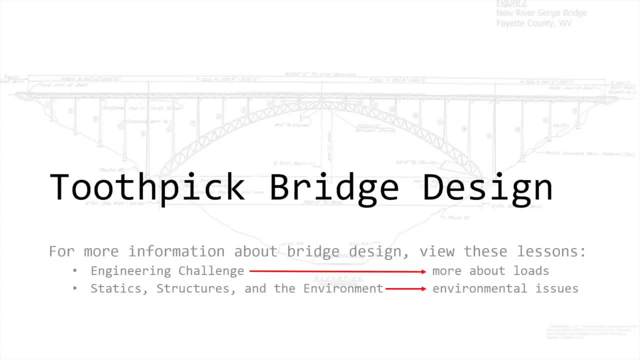 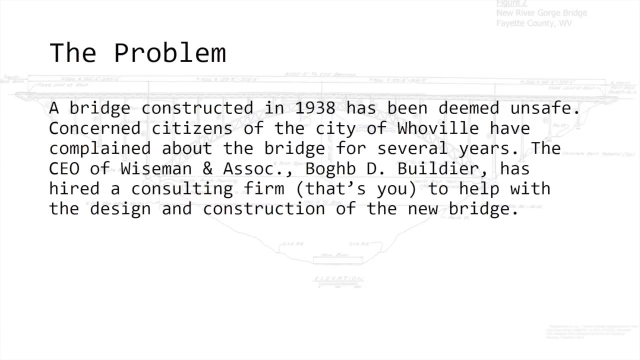 Now you can complete the toothpick bridge activity associated with this lesson. For more information about bridge design, you can also view the Engineering Challenge and Static Structures in the Environment video lectures. First, the problem statement: A bridge constructed in 1938 has been deemed unsafe. 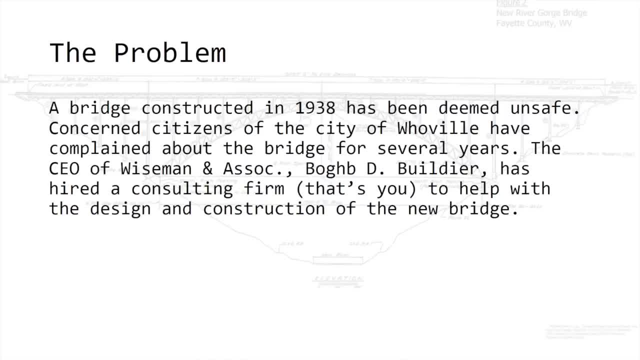 Concerned citizens of the city of Whoville have complained about the bridge for several years. The CEO of Wiseman & Associates, Bob D Builder, has hired a consulting firm- That's You- to help with the design and construction of the new bridge. 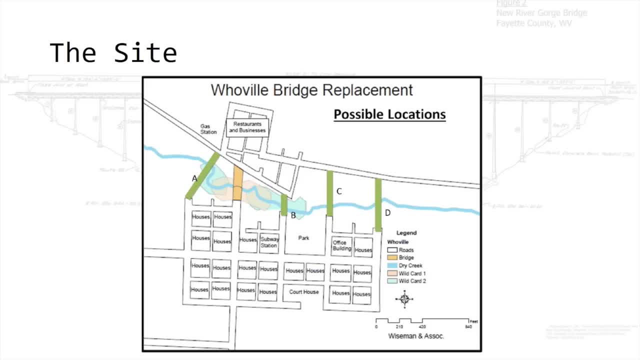 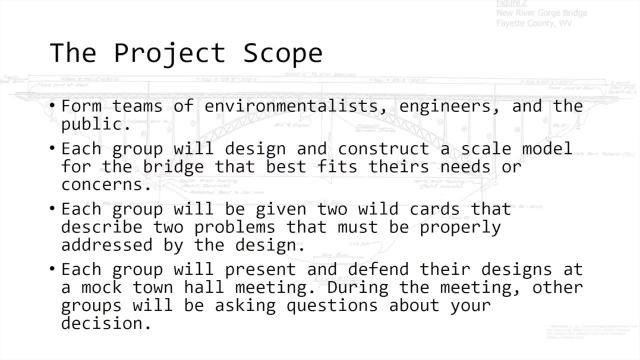 The site map has been provided to your firm, with the existing bridge shown in orange and the possible locations for the new bridge shown in green. The project scope involves forming teams of environmentalists, engineers and the public. From this point forward, you have three tasks to complete. 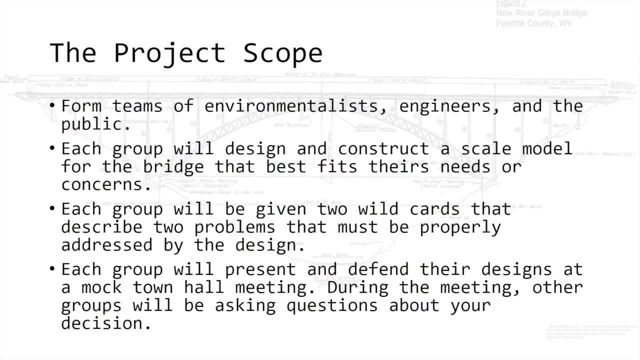 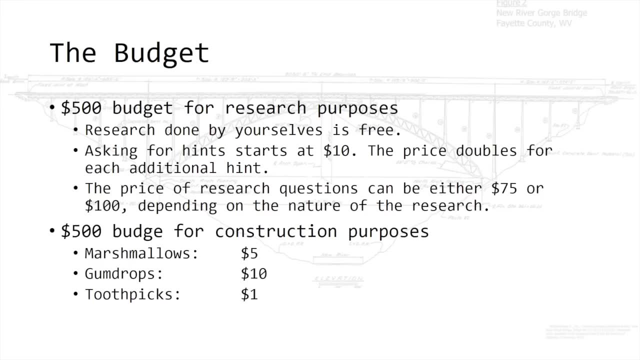 Each group will design and construct a scale model of the bridge that best suits their needs and concerns. Each group will need to address two wildcard problems with their design. Finally, each group will present and defend their design in a mock town hall meeting. The budget you will be able to work with. 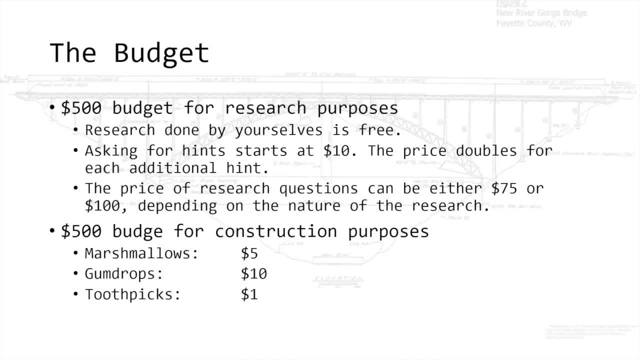 consists of $500 for research and another $500 for construction. Research and construction costs are outlined as follows: Research done by yourselves is free. Hints start at a price of $10 and the price doubles with each additional hint. Research questions can be $35 or $100,. 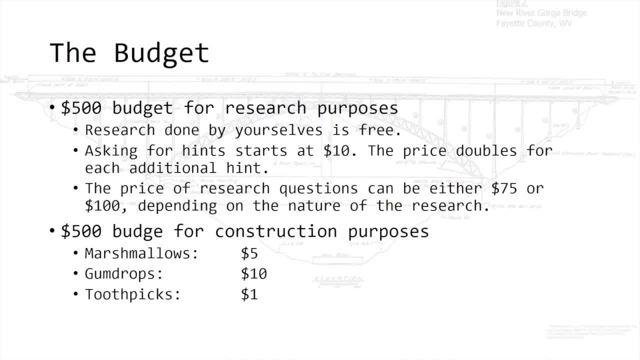 depending on the nature of the research, You can use marshmallows, gumdrops and toothpicks to construct your bridge. Marshmallows cost $5.. The cost of construction is $10.. Marshmallows cost $5,. gumdrops $10,. 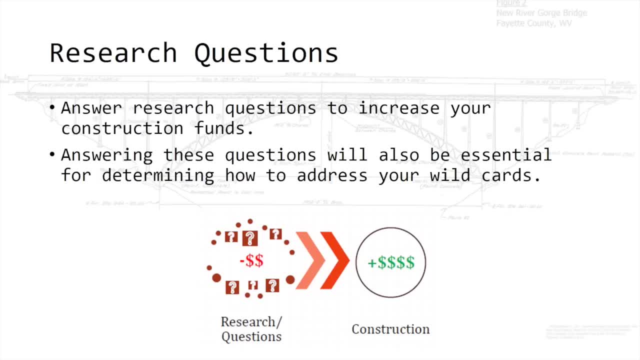 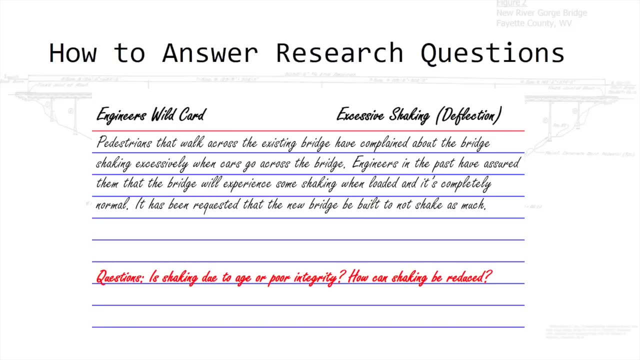 and toothpicks: $1.. Answering research questions can boost your construction funds while also helping you to solve your wildcard problems. We'll briefly discuss the criteria for answering research questions. Suppose this is a sample wildcard for engineers which deals with excessive shaking. Pedestrians that walk across the existing bridge have complained about the bridge shaking excessively when cars go across the bridge. Engineers in the past have assured them that the bridge will experience some shaking when loaded and it's completely normal. It has been requested that the new bridge be built. 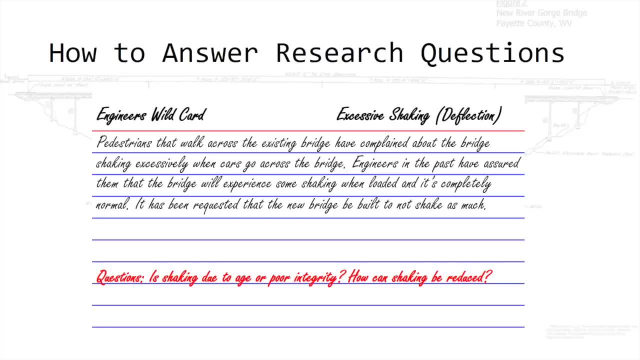 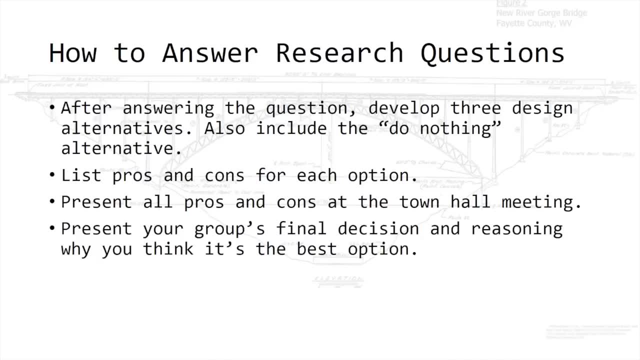 to not shake as much. The questions you must answer are: is shaking due to age or poor integrity, and how can shaking be reduced? Begin by answering the questions with cited sources, then proceed to develop three design alternatives. Also include the do-nothing alternative. 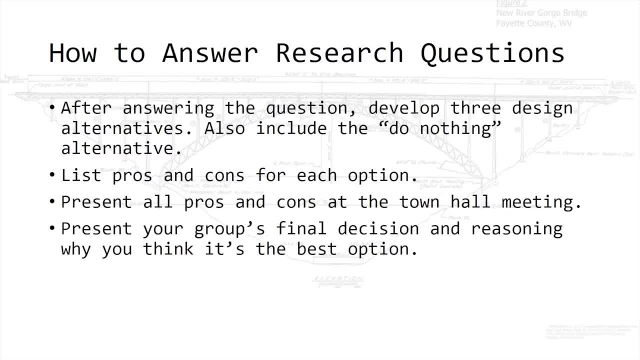 which means the existing conditions would be left as-is and no changes would be made. For each alternative list the pros and cons. You will present these pros and cons in the town hall meeting, along with your final decision and reasoning supporting your decision. 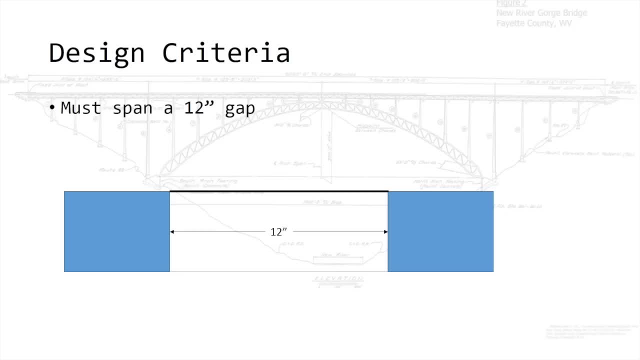 You also have some design constraints that must be taken into consideration. The bridge must have a 12-inch clear span between the abutments. The bridge must have a minimum height of 2 inches, But it cannot exceed a height of 8 inches. 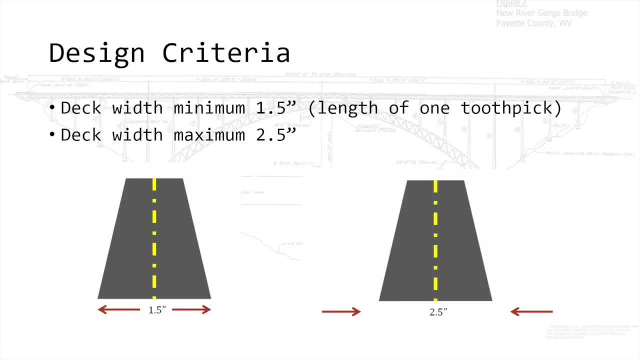 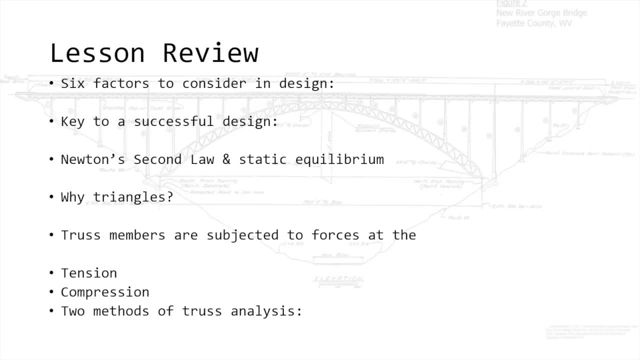 The deck width must be a minimum of 1.5 inches, but cannot exceed 2.5 inches. Before you begin the activity, let's review some of the key concepts covered in this lesson. Pause the video for a few minutes and try to fill in the answers before you view the answer key. 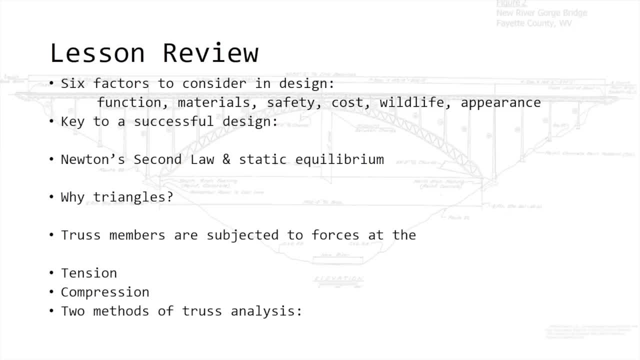 The six factors to consider in design are function, materials, safety, cost, wildlife and appearance. The key to a successful design is an adequate load transfer system. Newton's second law states that net force equals mass times acceleration. Static equilibrium is derived from this statement.